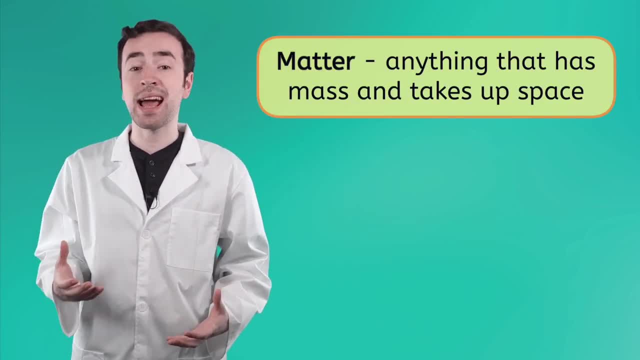 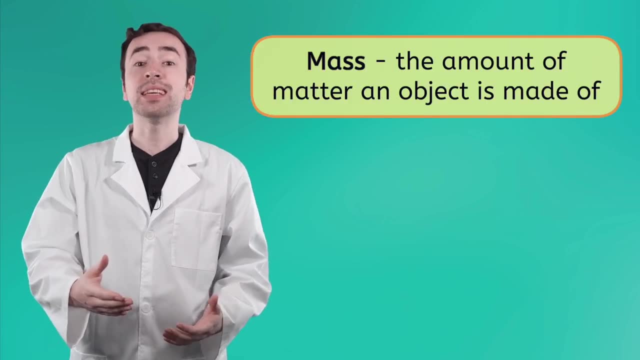 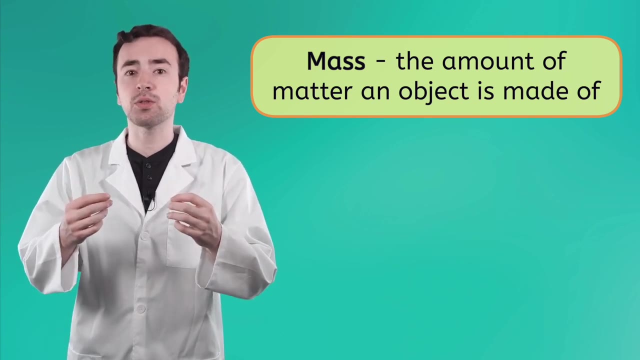 Matter simply describes anything that has mass and takes up space. So what does that mean? Well, let's break it down. Mass is the amount of matter that an object has or, more simply put, it's the amount of substance or stuff that's in something. 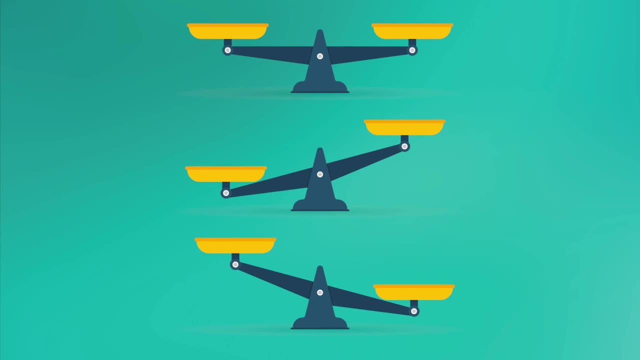 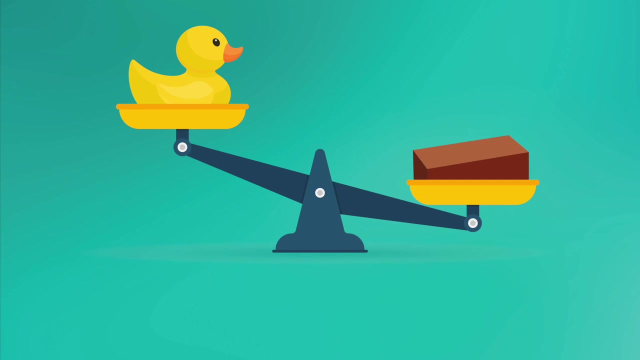 We can use a balance to compare the mass of two objects. If we put this rubber ducky on one side of the balance and this brick on the other side, we can see the brick has more mass than the rubber duck because its side of the balance is lower. Which do you think has more mass? a dictionary. 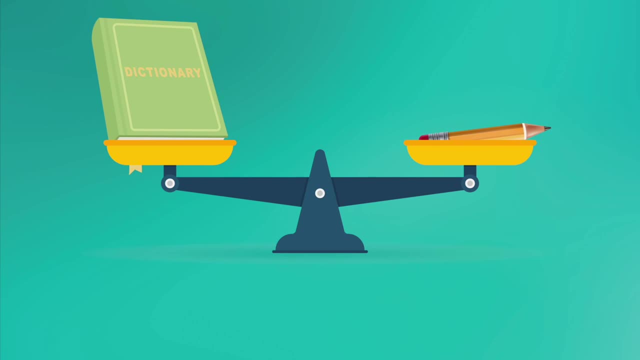 or a pencil. If you said the dictionary, that's right. The dictionary literally means that tener, The abstract word for deter, does not have any more point than a particle, but it has more matter or substance inside of it compared to the pencil, so it has. 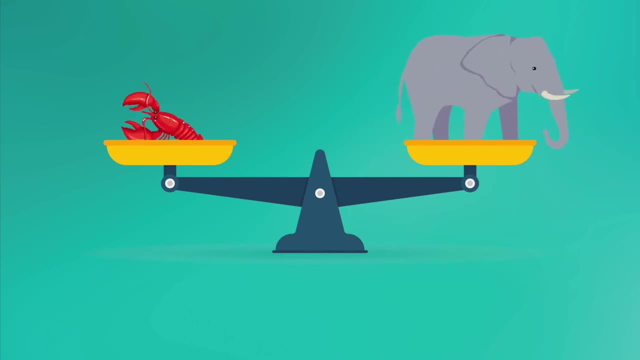 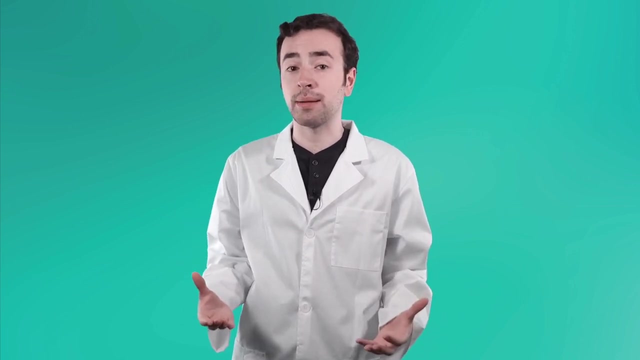 more mass. How about these? Which do you think has more mass? a lobster or an elephant? Yeah, definitely the elephant. Now, you might think that a bigger object has more mass in it, and that's true sometimes, like with the lobster and the elephant. 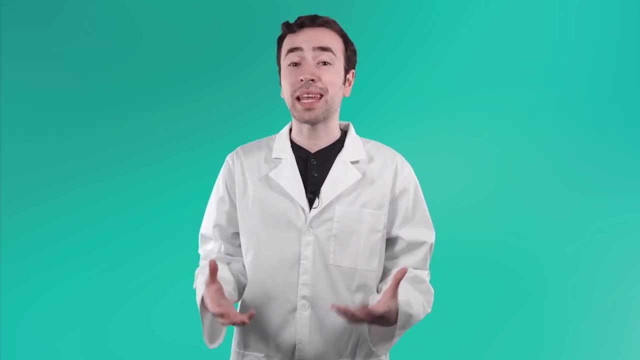 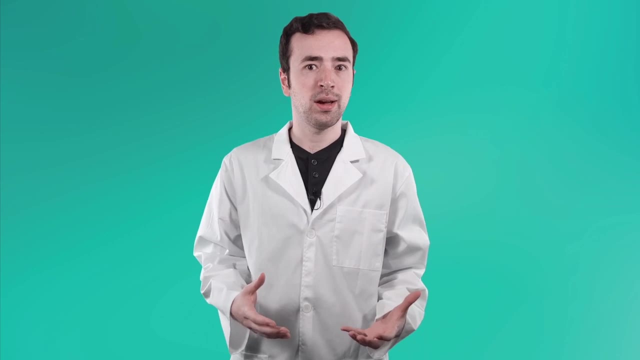 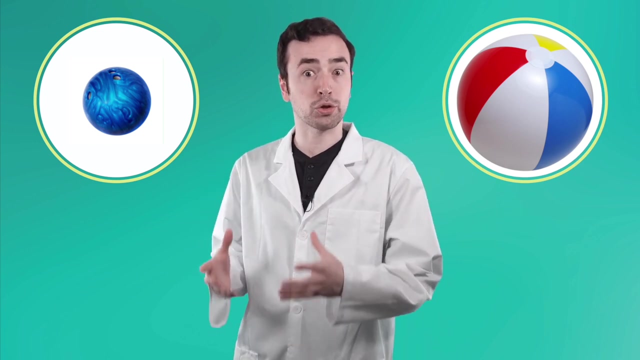 true all of the time. In fact, objects with the same size can have totally different masses, and smaller objects can even have more mass than bigger ones. For example, a bowling ball is smaller than a beach ball, but the bowling ball has much more mass. Similarly, a shoebox that's. 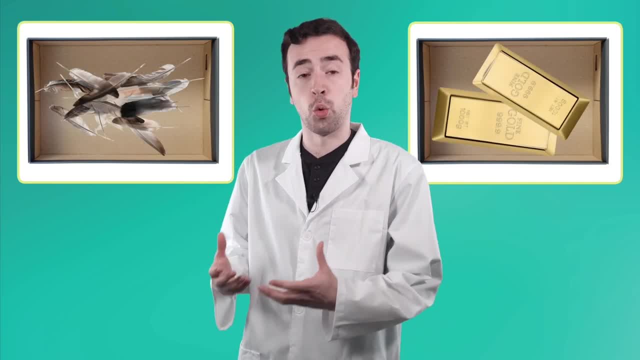 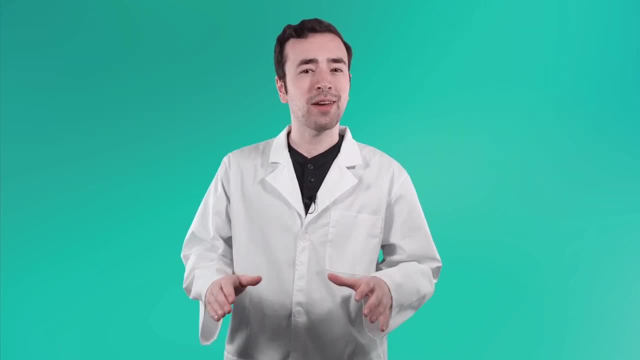 full of feathers would be the same size as a shoebox that's full of gold bars, but I think you could tell which one of these has more mass too. Now that we're starting to get the hang of it, why don't you take this time to pause the video here and try some more examples on your own? 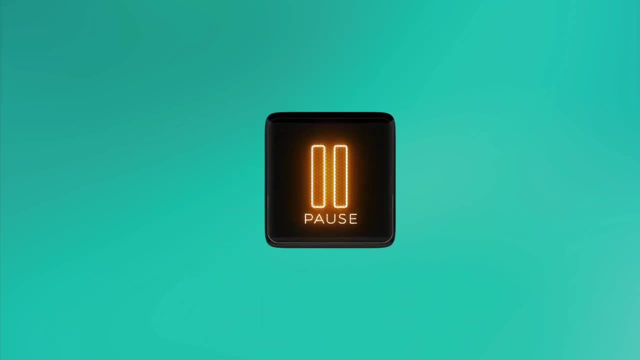 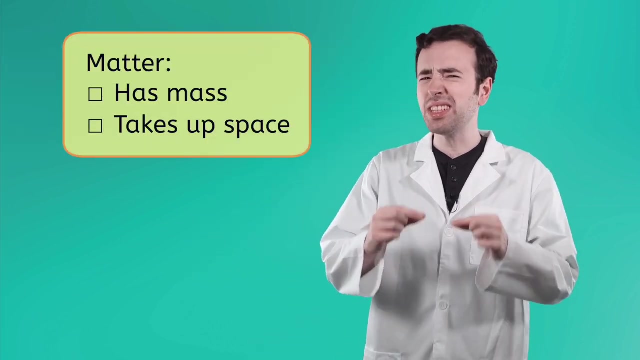 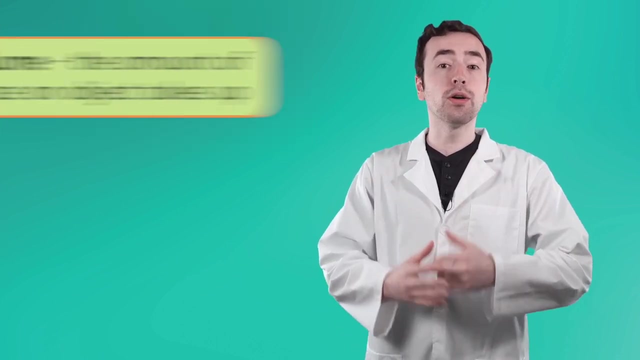 in your guided notes. So now we know that for something to be matter it has to have at least a little mass. but we also said that for something to be matter it has to take up space. Volume is the term we use to describe the amount. of mass that we have in our body. So if we have a lot of mass, we have to have at least a little amount of mass. So if we have a lot of mass, we have to have at least a little amount of mass. 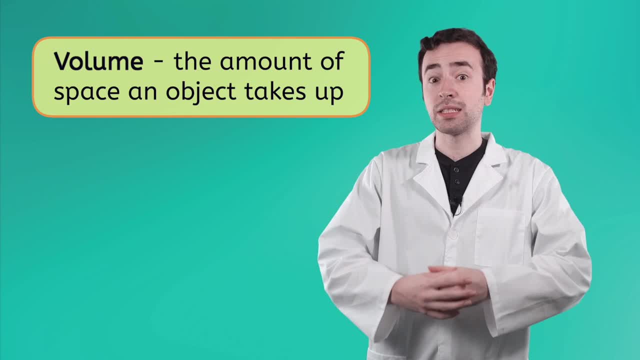 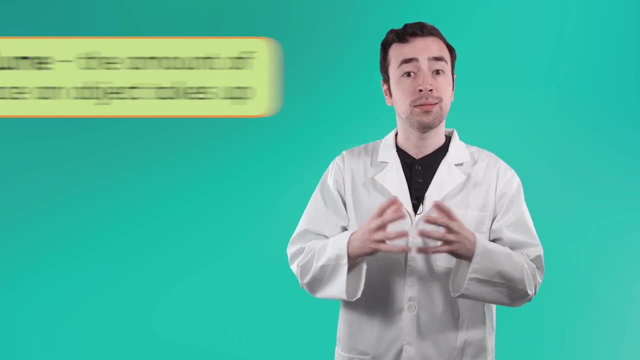 So if we have a lot of mass, we have to have at least a little amount of space that an object takes up. If something has more volume, then it takes up more space. If something has less volume, it takes up less. Now that we know what volume is, which do you think has more volume This apple? 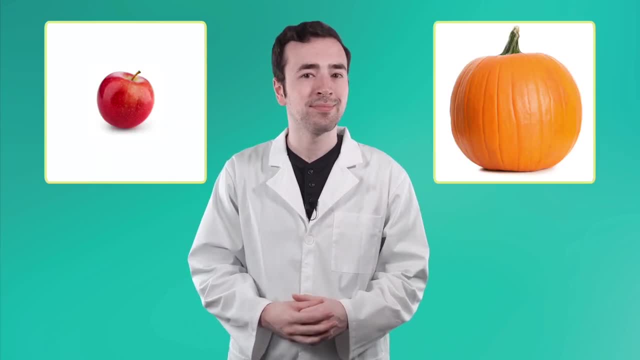 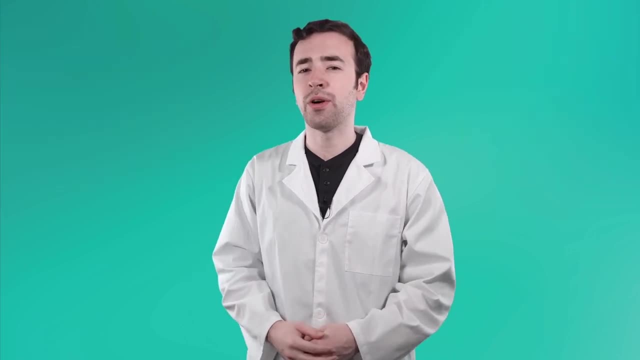 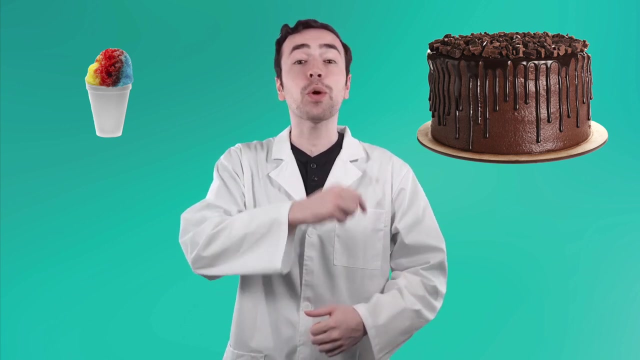 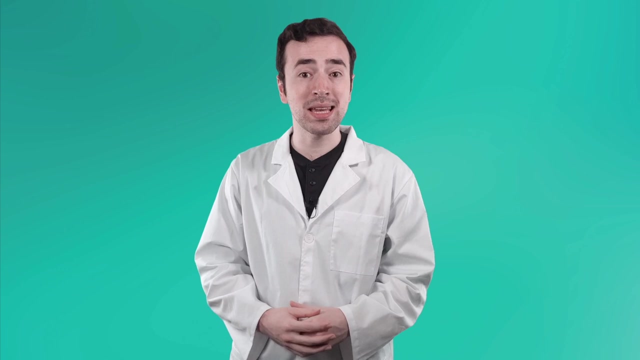 or this pumpkin. The pumpkin has more volume because it takes up more space, Which has more volume. This snow cone. or this chocolate cake- If you said the cake, you're right. Remember, just because an object has more volume, that doesn't necessarily mean it has more mass. Pause the video here and try out a few more. 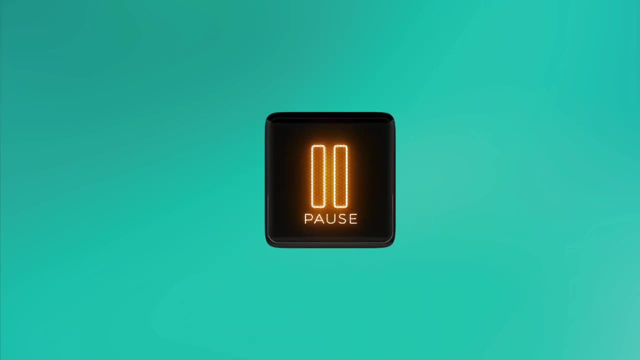 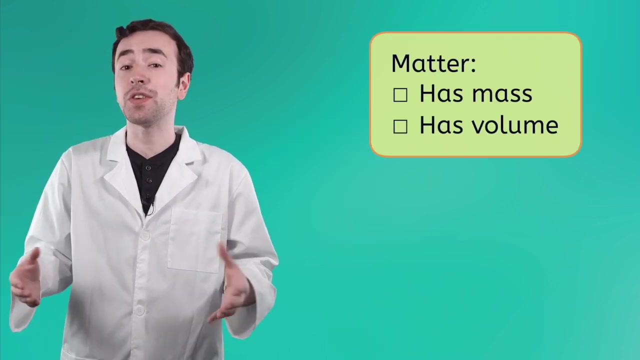 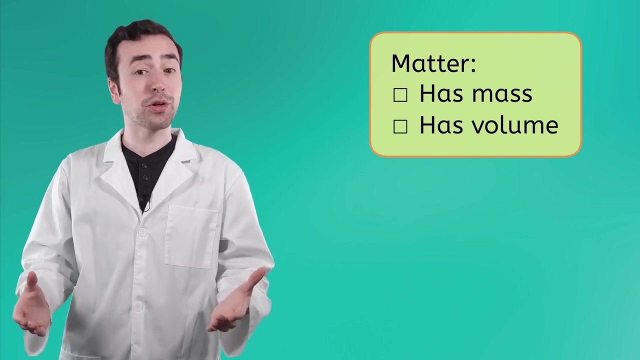 examples in your guided notes. Okay, so now we know, regardless of how much of each it has. if something has mass and it has volume, then it is matter. Let's take a look at some examples now to try to figure out what is and isn't. 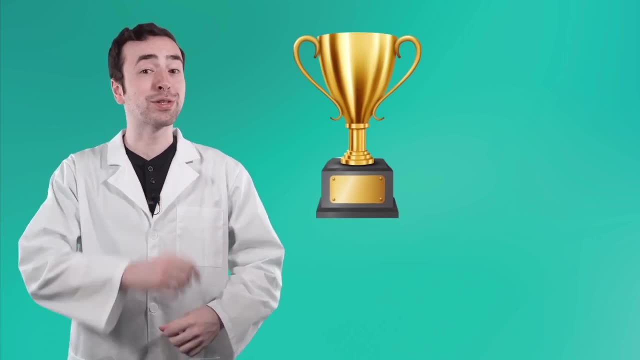 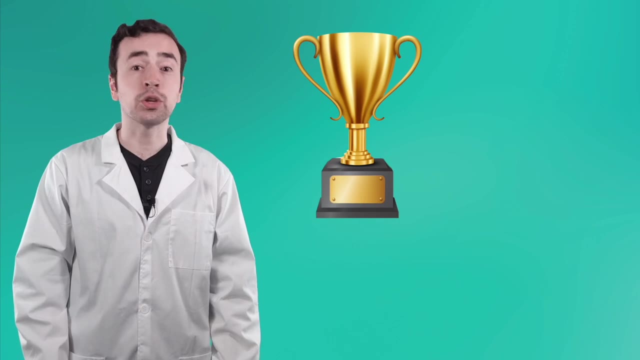 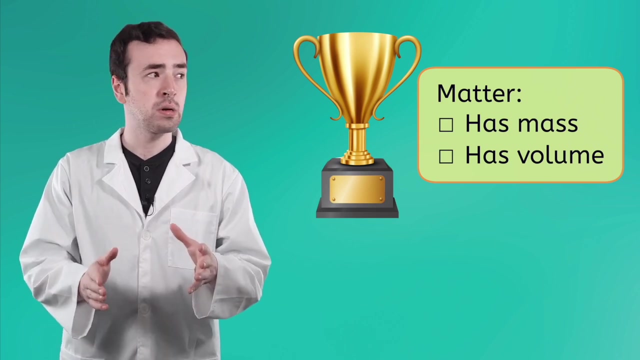 matter. My sister's soccer team won this awesome gold trophy the other day. Is it matter? Remember to find out. if something is matter, you can ask yourself two questions: Does it have mass and does it have volume? So, is this trophy matter? Well, the trophy has mass because it. 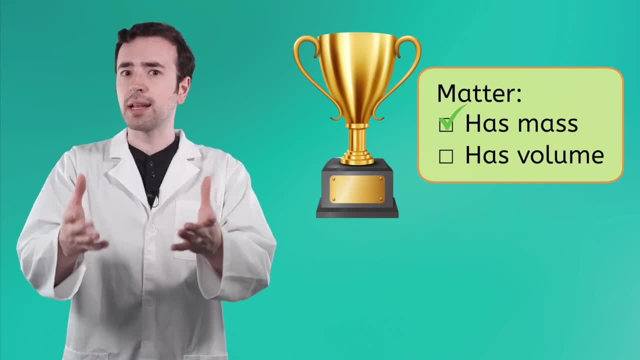 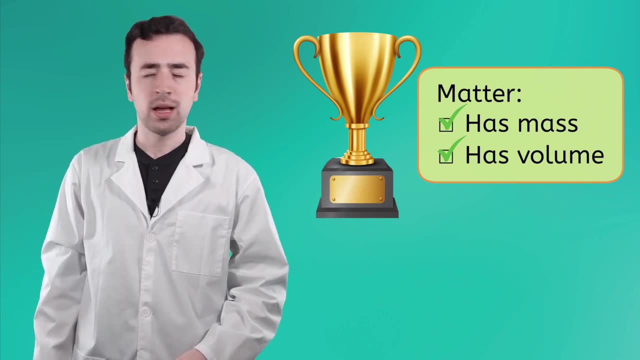 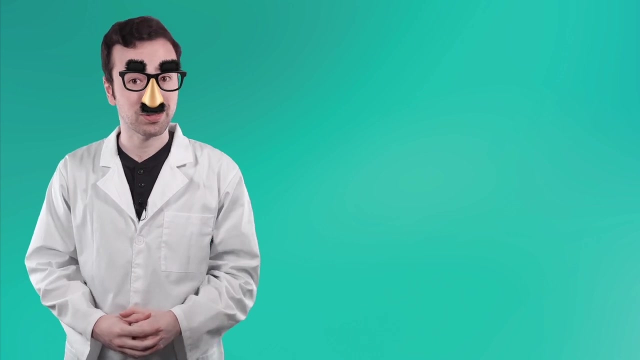 has substance, it's made of stuff and it has volume because it takes up space. Therefore, this trophy is definitely matter. What about these awesome wacky glasses I have? Are they matter? Remember to ask yourself the two questions. Yep, the glasses have mass and they take up. 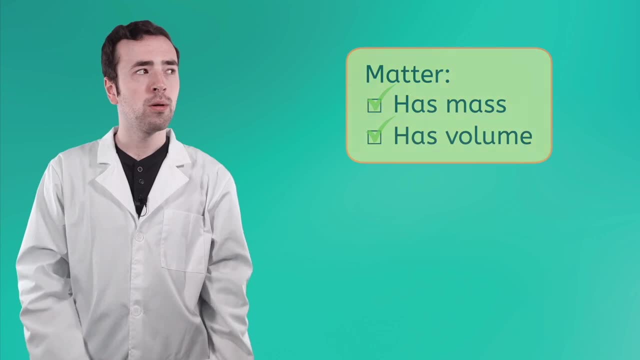 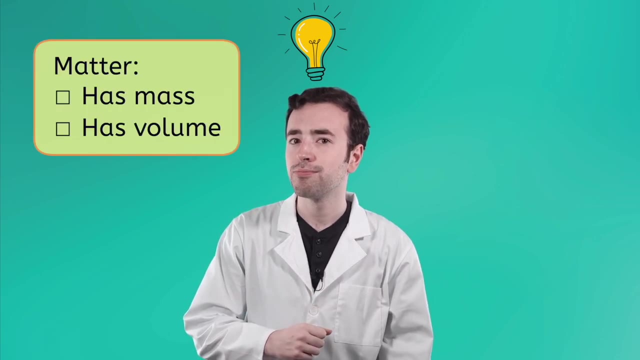 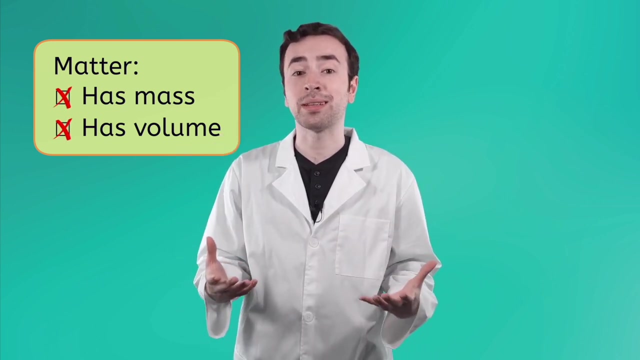 space. so they are matter. Oh, I have an idea. Is my idea matter? Nope, my idea does not have mass and it doesn't take up space, so as good as it is, it is not matter. It's a shame too. This light bulb is really. 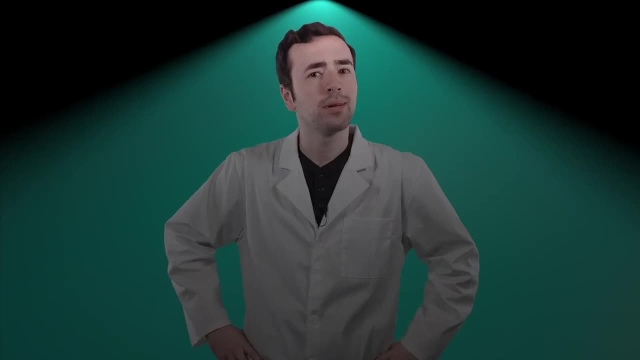 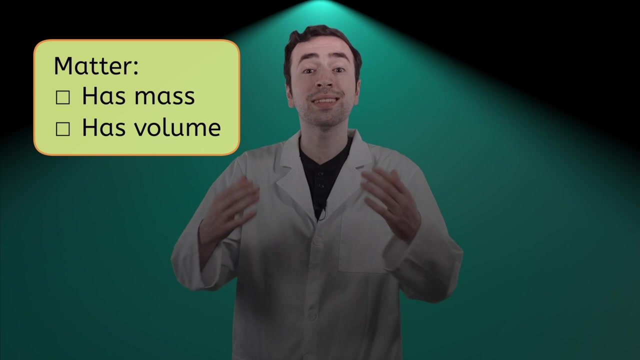 cool, It's giving off a really pretty light. Is light matter? No, No, No, No, No, No. Light doesn't have mass and it doesn't take up space. Therefore, light is not matter. Okay, here's a tough one for you. 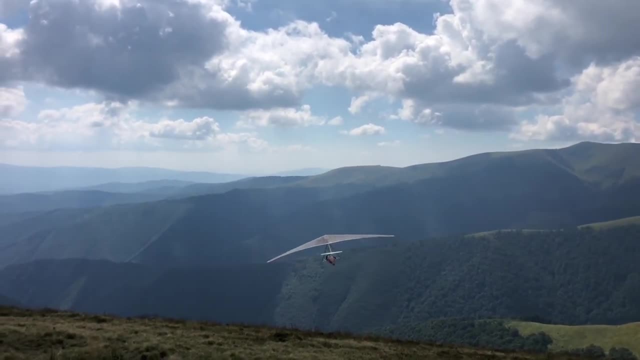 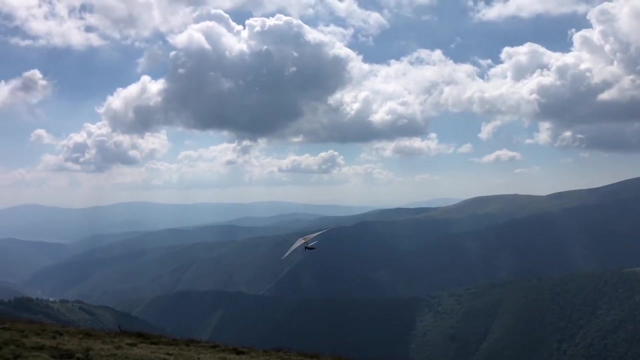 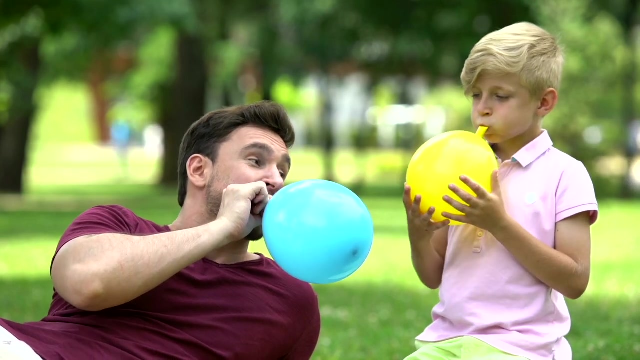 Is air matter? Even though it can be hard to tell, air has mass and volume, so it is made of matter. Imagine blowing up a balloon. As you blow into it, the balloon expands. Air is filling the space inside of it, which shows that it has volume. 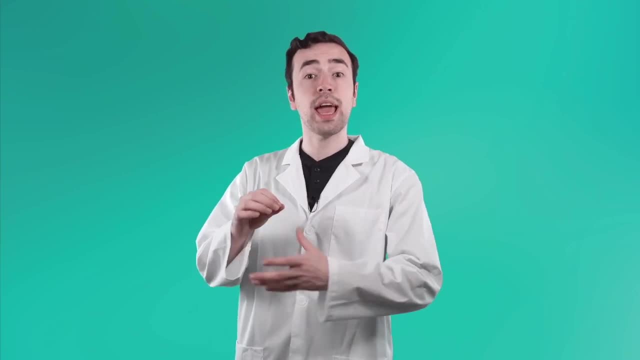 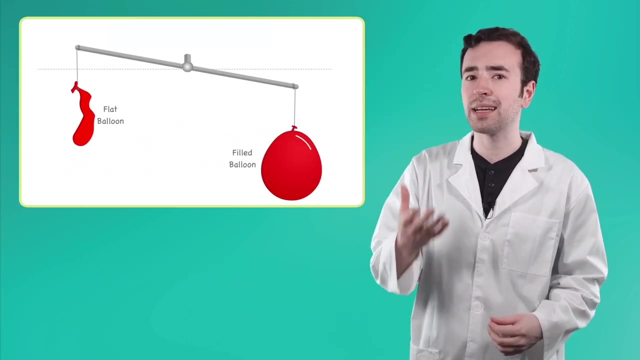 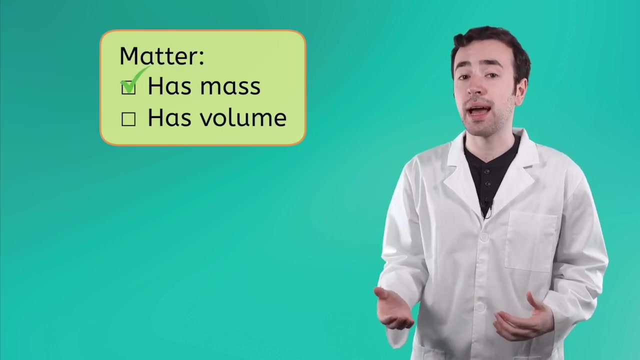 Air also has mass. If you take a filled balloon and put it on a balance with an empty balloon, you will find that the filled balloon has more mass, that must be coming from the air. So since air has mass and volume, air and all gases in fact, are matter. 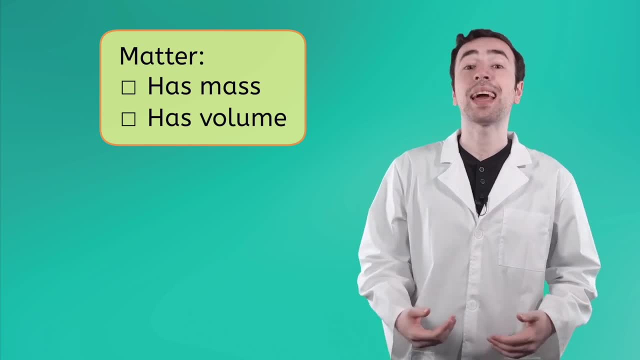 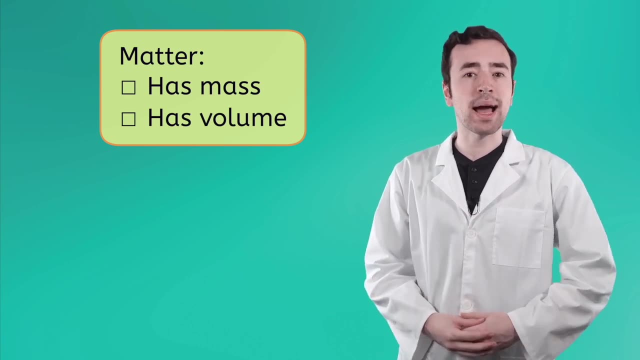 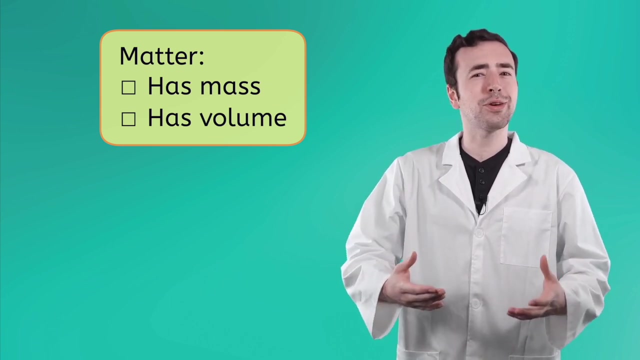 Okay, We now know that matter is anything that has mass and volume. Volume is the amount of space an object takes up and mass is the amount of matter or substance or stuff the object is made of. But what is all that stuff exactly? 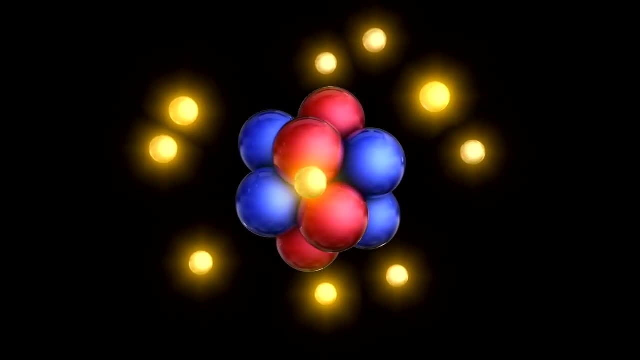 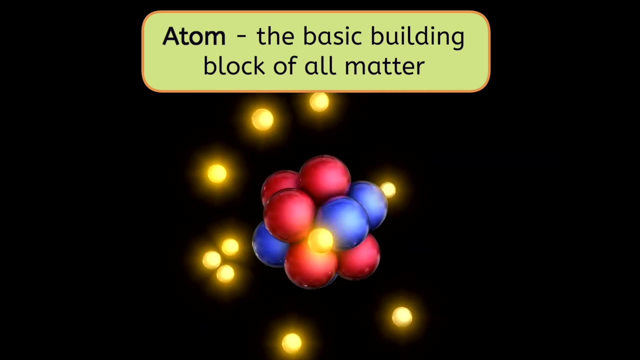 All matter in the universe is made of atoms. Atoms are the most basic building blocks of matter, and they are the most basic building blocks of matter. Atoms are far too small to observe with our own eyes. They are so tiny it can be difficult to wrap your head around it. 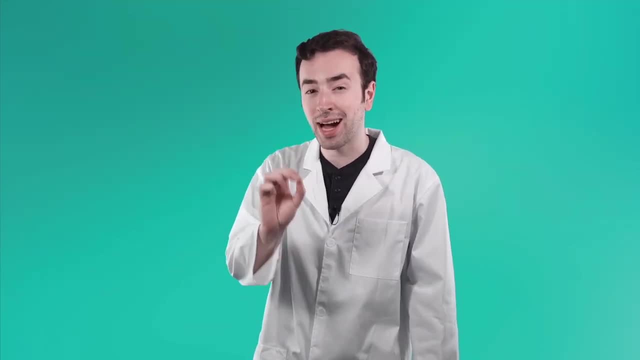 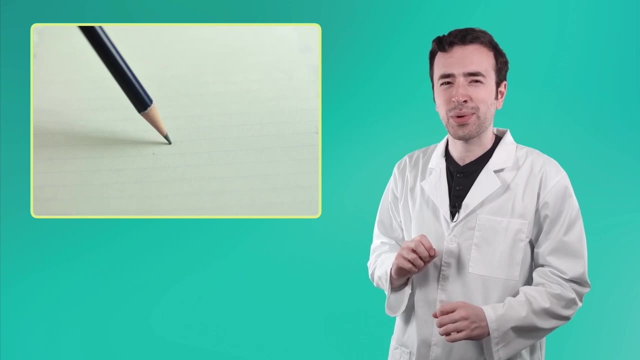 Let's try to visualize just how tiny an atom is. I want you to take a pencil or a pen and draw a teeny tiny dot on your paper, like the tiniest dot you can make. Just go See how tiny that dot is. 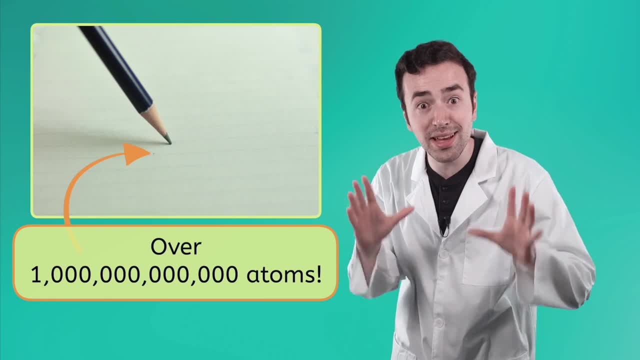 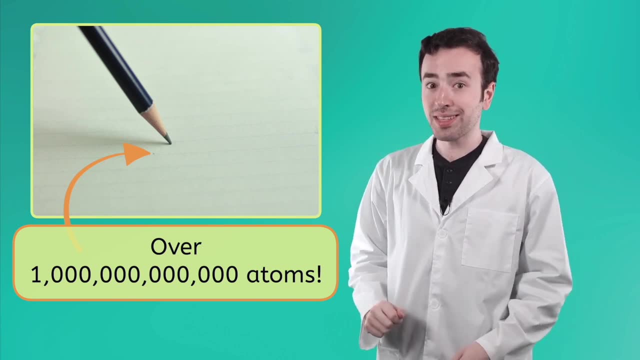